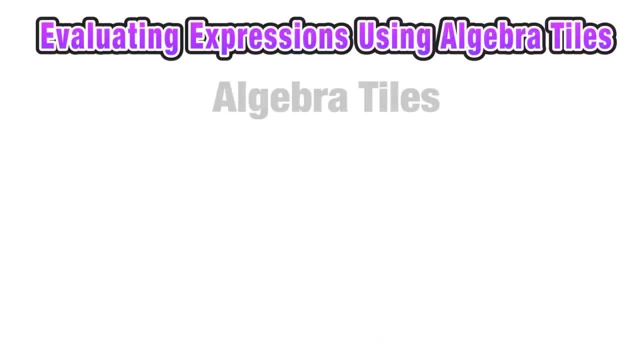 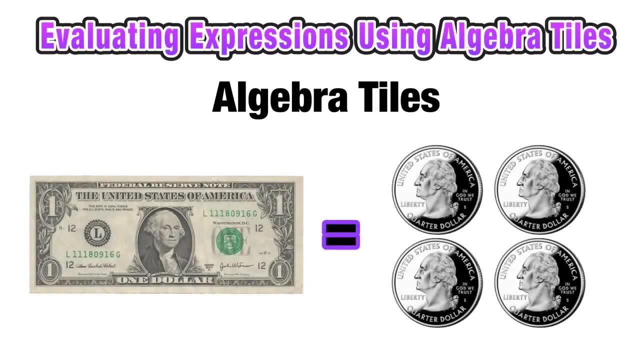 8x plus 14.. So before we start using algebra tiles, let's think about how one dollar is the same thing as four quarters, So we can think of a one dollar bill as a representation of four coins that are each worth 25 cents. 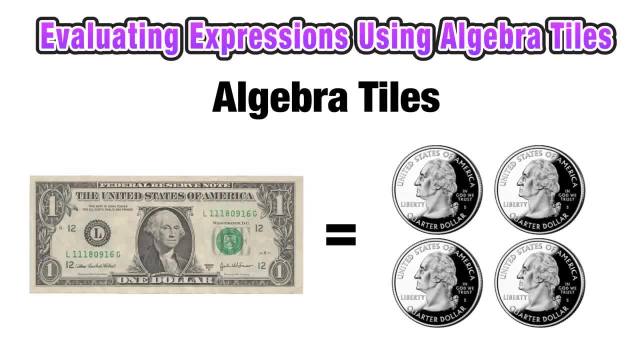 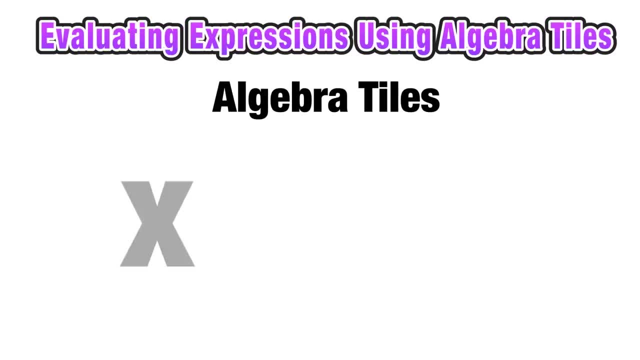 Algebra tiles work in a very similar way. so now we're going to go ahead and extend this thinking to evaluating algebraic expressions. So to represent our variable x, we are going to use an algebra tile that is a green rectangle. If we wanted to represent 2x, we would need two green rectangles. 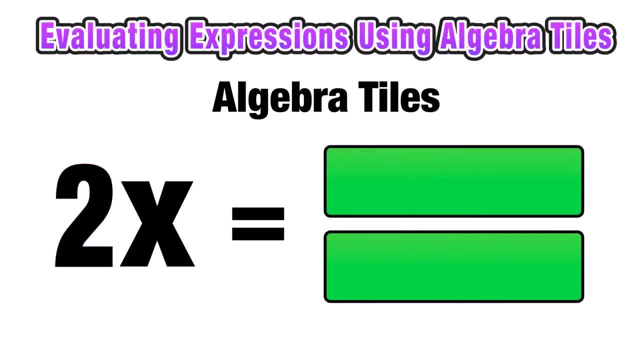 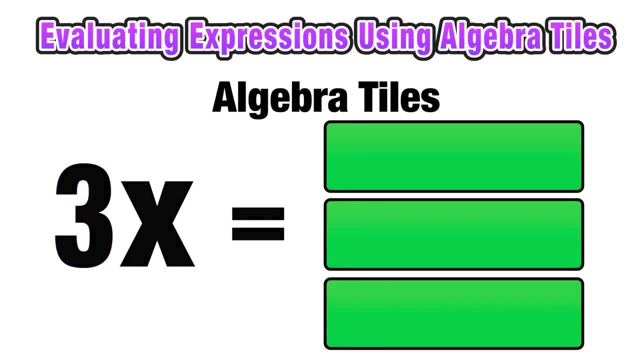 So we would need two green rectangles So to represent our variable x, we are going to use an algebra tile that is a green rectangle. If we wanted to represent 3x, we would need three rectangles, and so on and so forth. 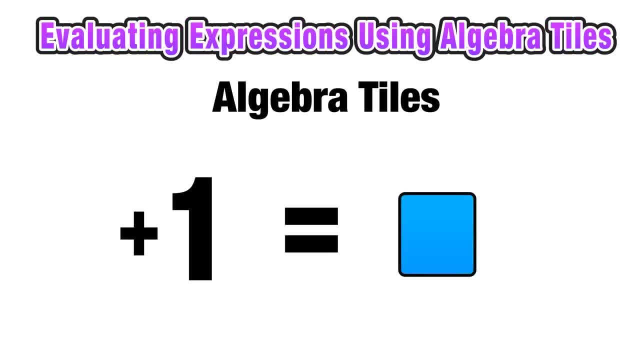 Now, a value of positive 1 is represented by a blue square algebra tile. So if we wanted to represent positive 2, we would use two blue squares. If we wanted to represent positive 5, we would use five blue squares. So it's pretty simple here. 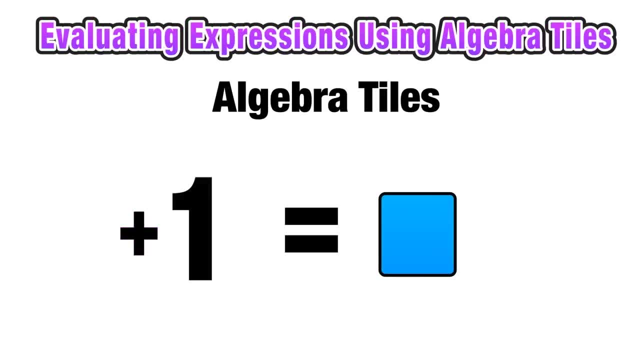 Each one represents positive 1.. However, If the sign was negative, So if we wanted to represent negative 1, we would have to use a red square. So to represent negative 3, we would use three red squares. If we wanted to represent negative 6, we would use six red squares. 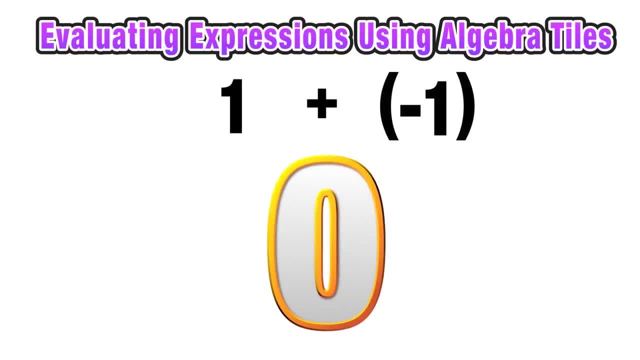 Now we know that positive 1 plus a negative 1 is equal to zero. Basically, they cancel each other out. So, in terms of algebra tiles, Positive 1 is represented by one blue square, Negative 1 is represented by one red square. 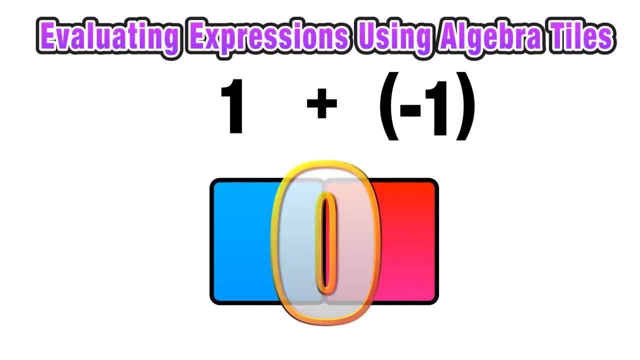 And again, if I combine those two, One plus negative 1 will equal zero. So in this case, with algebra tiles, they will cancel each other out and effectively disappear. So, for example, if we wanted to use algebra tiles to represent 7 minus 3.. 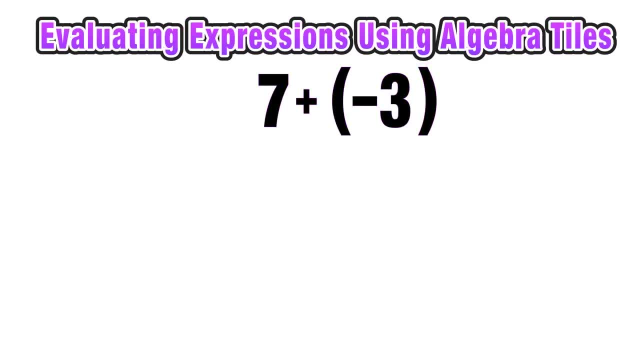 We can rewrite this as 7 plus negative 3 and then model it using tiles. I'll replace positive 7. With 7 blue squares And I'll replace negative 3 with 3 red squares. Now I can pair up the combos of one blue square and one red square when I combine this. 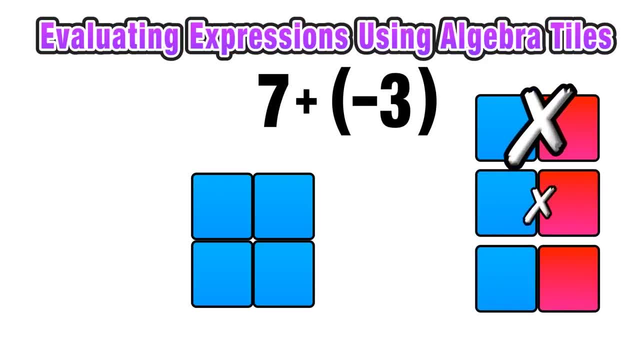 So by pairing those up, I know that a combo of positive 1 and negative 1 is going to become zero and cancel out, And what I'm left with here is 4 blue squares. So I can say that 7 plus negative 3 is equal to positive 4.. 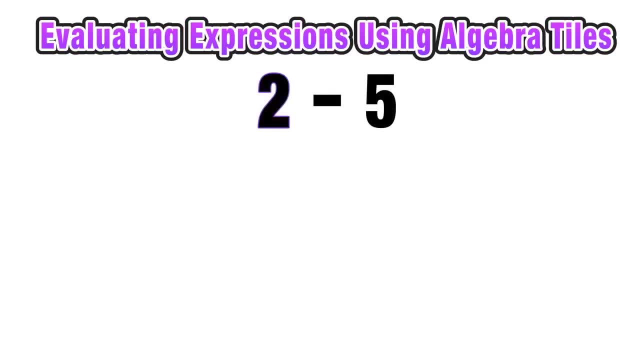 Oh yeah, What about 2 minus 5?? I can represent positive 2 with 2 blue squares And negative 5 with 5 red squares. Again, I can pair up any combos of a blue and a red square Which will cancel out. 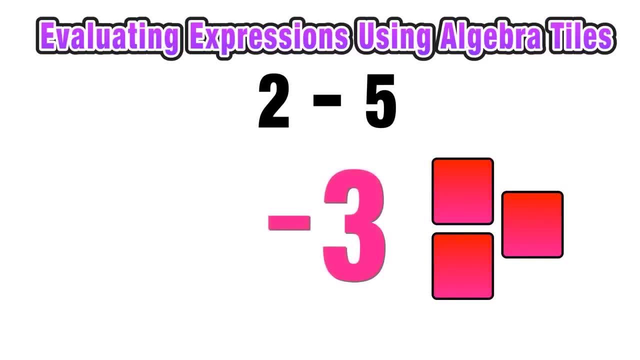 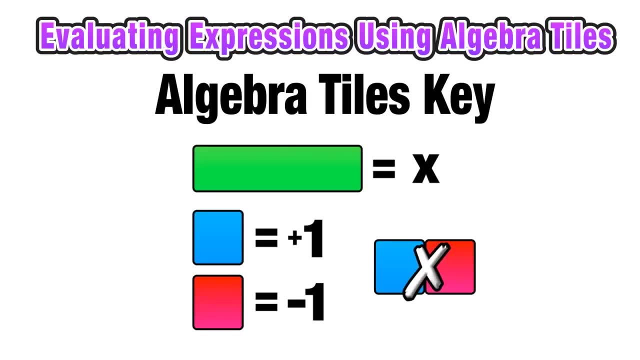 And what I'm left with is 3 red squares. So I can say that 2 minus 5 is equal to negative 3.. So let's use this key to make sure that we're familiar with How to use algebra tiles. Remember that the green rectangle represents x. 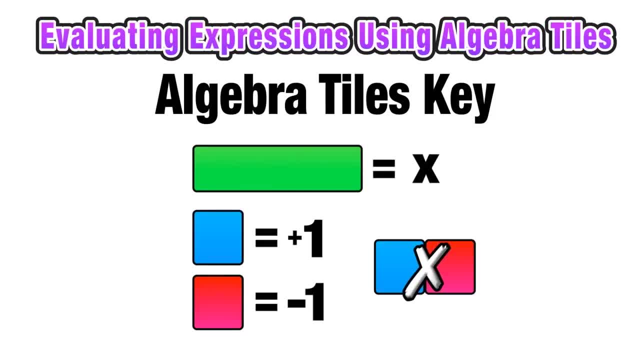 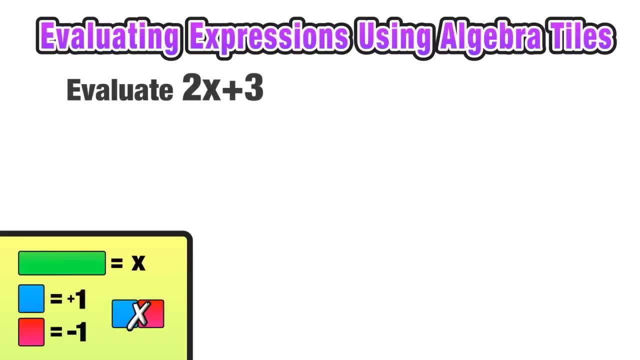 A blue square represents positive 1.. A red square represents negative, 1. And a combination of one blue and one red square, One plus negative 1, would equal zero. So they cancel each other out. Okay. so let's go ahead now and evaluate some expressions using those algebra tiles. 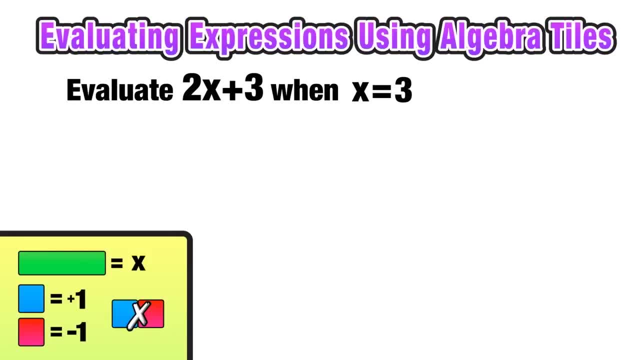 So our first example says to evaluate 2x plus 3 when x is equal to 3.. First We want to model the expression 2x plus 3 using algebra tiles. So first we lay out two x's And then we lay out positive 3.. 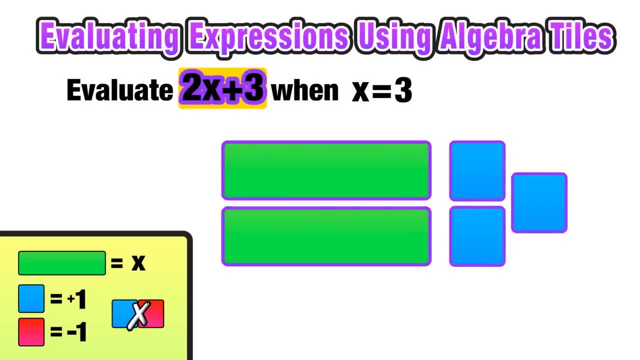 So these algebra tiles now represent that expression: 2x plus 3.. The next step is to evaluate this expression for when x is equal to 3.. So I have to replace each x with a value of 3.. In this case, with 3 blue squares.